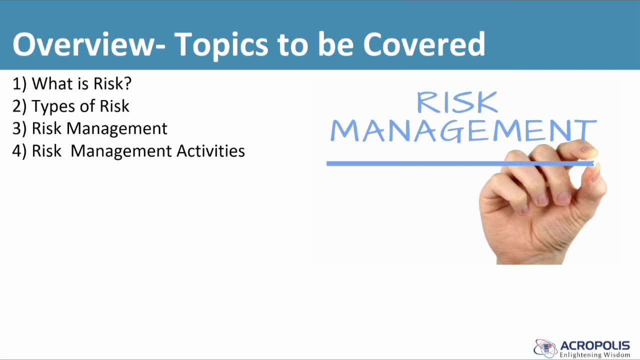 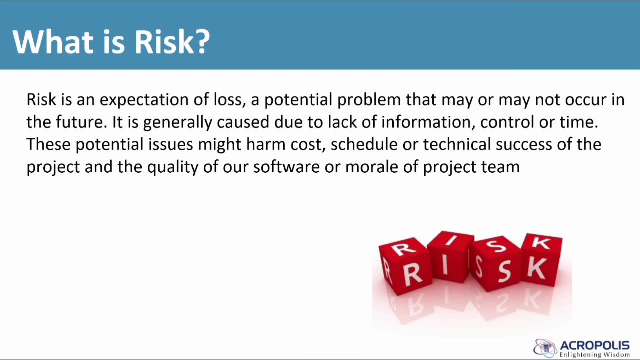 To avoid risk. So let us start. what is risk? So in day to day life, we always come to know. like we always use the term risk, We always say, yeah, this is risk, or if you are doing something, then there may be risk. So in software development as well, risk is nothing that much different. It is also expectation of loss or potential problem that may or may not occur in future, And generally it is caused due to lack of information or control, or 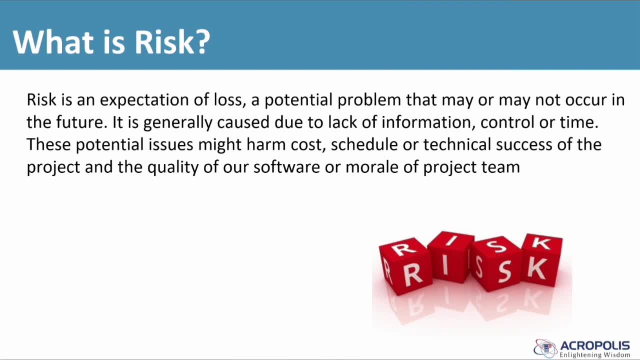 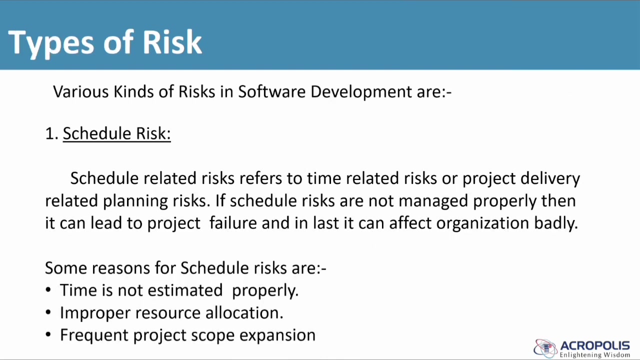 time And the potential issues. that in risk is that it can harm cost, schedule or technical success of the project And it also like take in risk It can also affect the quality of software and also the morale of the project team. So hope you know what is risk and let us move ahead and see what are the types of risk in software development Also. the first one is schedule risk. 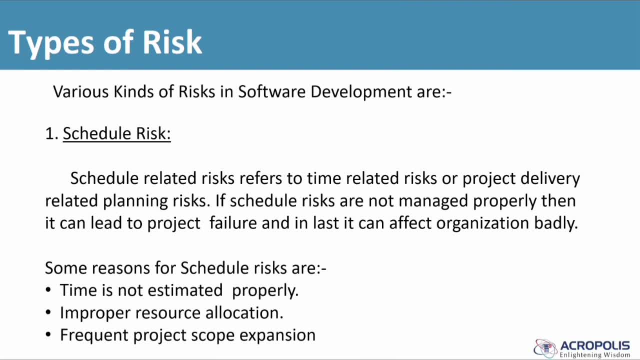 In schedule risk refer to the time related risk or project-related planning risk. Okay, that means if we are not managing the time properly, then it may lead to schedule risk And it can affect. if it is not manage properly, than it can cause project failure as well as it can affect organization as well. So there is some regions that can. that is reason for schedule risk are a time is not. 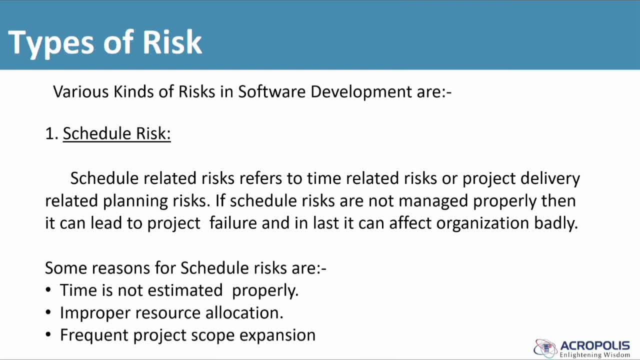 estimated properly, Or if resource is not allocated properly, or if we are doing expense on a project, very frequently effects like, if you like, if there is some project expansion, like if there is a project, is scope and we are expanding in on very frequent basis and it may lead to schedule risk. so now the next one we have is budget risk and we 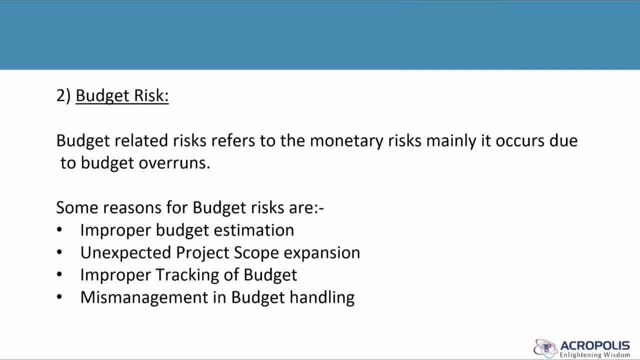 also know how much budget is important. so the it refers to the monetary risk, like if it, if the budget is over running, if you don't have proper budget, then it will lead to a budget risk. so the reasons that is like if. like already told, if we have improper budget estimation or if scope of project is. 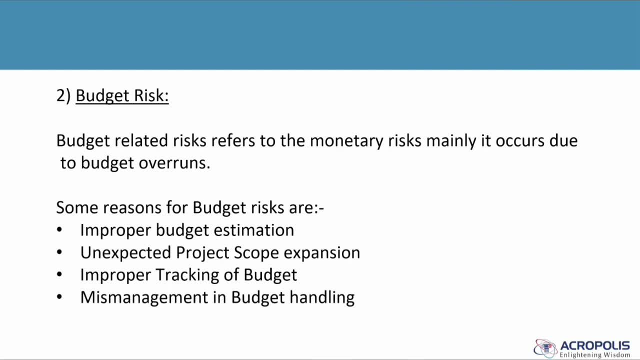 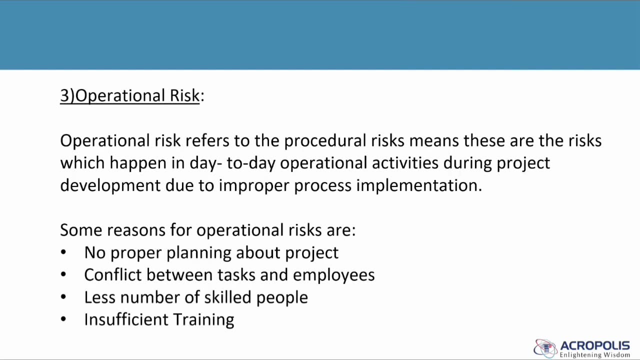 expanded unexpectedly and if we are not tracking the budget properly or if you are handling the budget not carefully, then it may lead to budget risk. thank you. now the next one we have is operational risk. operational risk are the risk which uh happen in day-to-day operation and like if we are not following the proper process or if, like, there is. 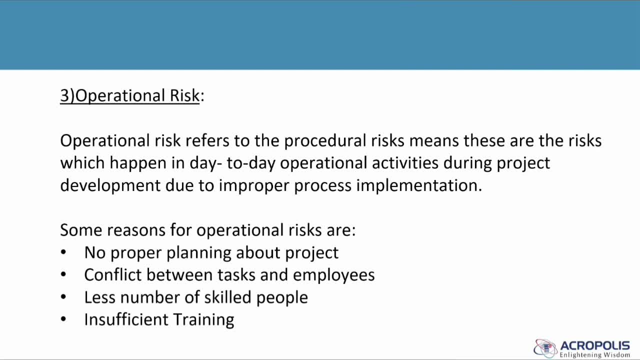 improper process implementation, then it may lead to operational risk, and the reasons uh for operational risk are if we have not made proper planning about project and uh another one is if we have like conflict between task and employers. and the last but not least, it is very important. 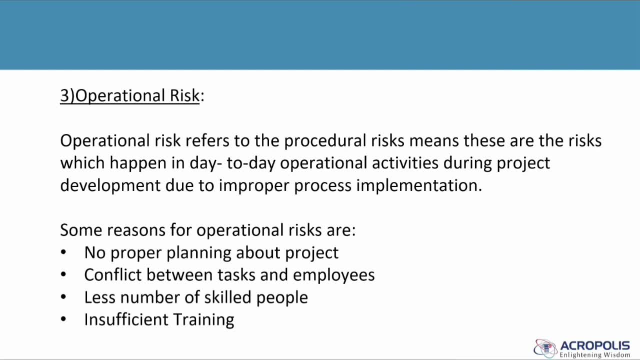 in any organization to have a good amount of skilled people. if the number of skilled people are not there, then the chances of operational risk is always high and uh, for that, what we can generally do, like we we can have as much skilled people we can, and also it is very much important. 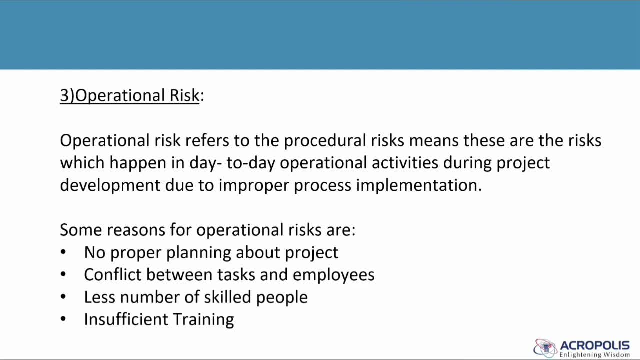 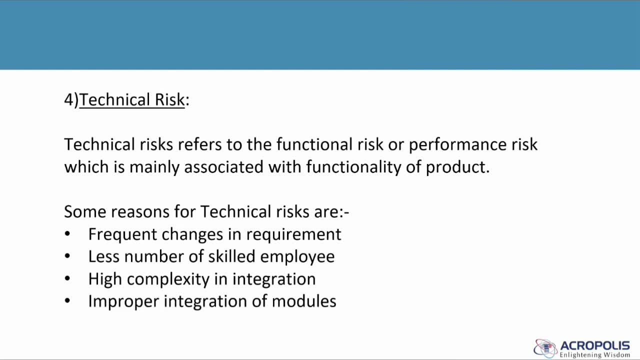 to uh give sufficient training before uh doing any project. and uh. the next one is technical risk. it is more related to the functional risk or performance risk. uh, it is mainly associated with the functionality of that product, and the reasons uh behind the technical risk are frequent changes in requirement. if we are changing the requirements, 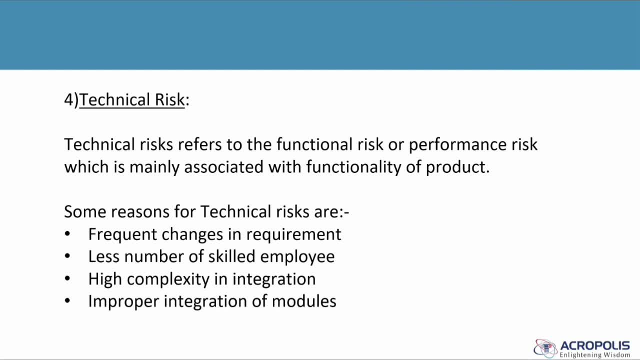 very frequently and uh also, uh, the same reason we have is, uh like, if you don't have a skilled employer, or the number of is called skilled employees very less, and uh like, uh, generally what we do in uh project, uh, we just break it into modules, okay, uh, so like, if there is a high 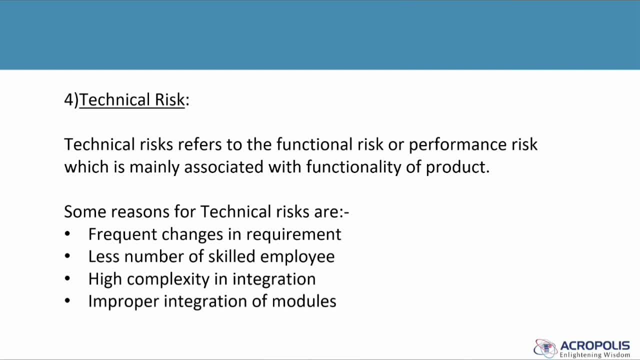 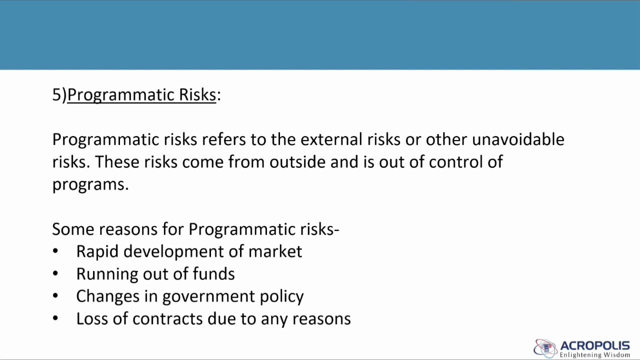 complexity integration, like if you develop the modules correctly, but uh, if you're not. uh like integrating it in correct manner, or like the. if integration is very complex, then it may lead to technical risk. now the next one is programmatic risk, and it is something that it is unavoidable. 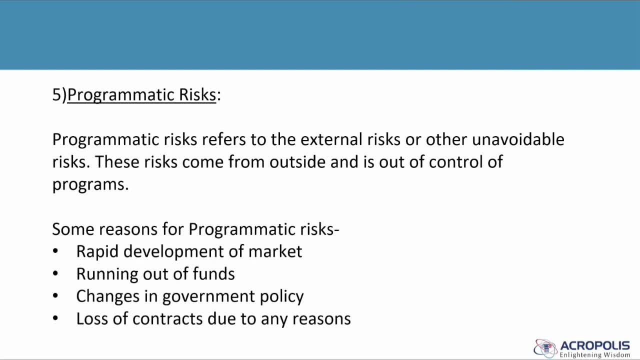 and it is generally external risk. it comes from outside and it is out of control. it's, it is out of control. uh, the reason behind it is like if there is a rapid development of market, so it can happen anytime. so it may lead to programmatic risk and also the running out. 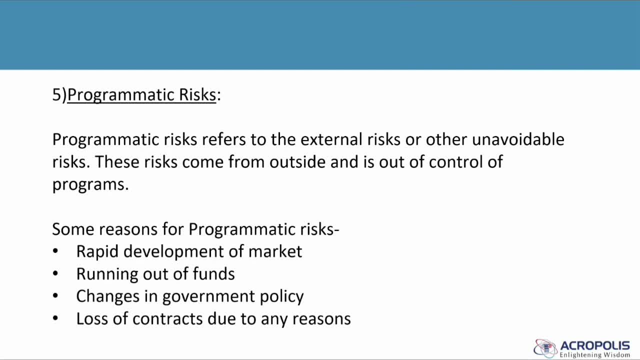 of fund is also, uh, a type of programmatic risk and it may also lead to programmatic risk and, uh like, changes in government policy can also affect or loss of contract is also a reason behind that. okay, so now we know what are risk and the types of risks. now let us move ahead. 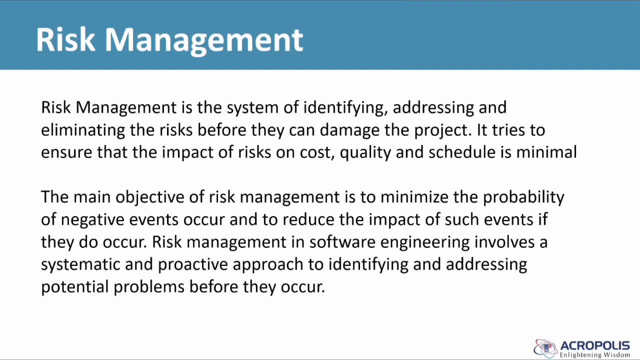 and see what is risk management, uh. so risk management is a system of identifying, addressing and eliminating the risk before they can damage the product. it is always better, uh, it is always better to know uh risk at earlier stage, as if we know it in earlier stage, then it always uh, we can. 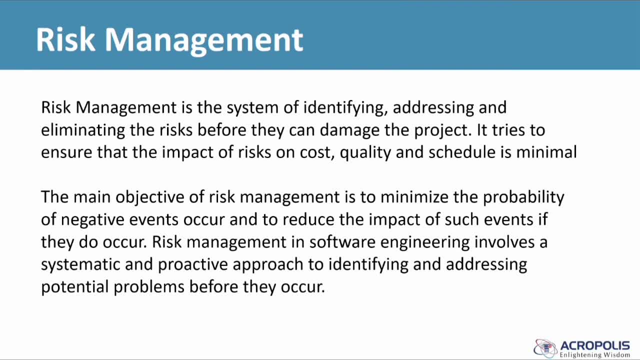 ensure that the impact of risk, of cost- risk on cost- is less and the quality is uh like better, right? so the main objective of risk management is to minimize the probability of the negative events that is occurring and uh, and also it reduces the impact of event if it is happening. 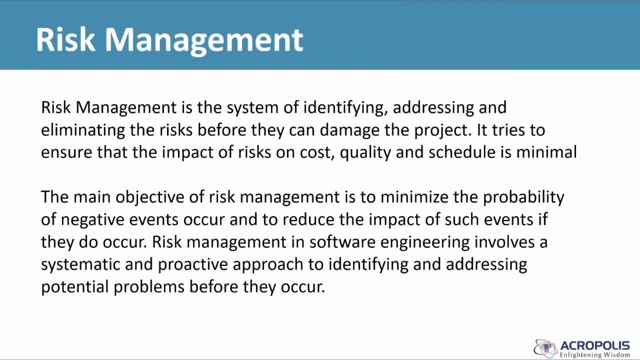 then it also tries to reduce the impact of that. so what we generally do, uh, we will see in later stage. uh, what we generally do, uh, we just like take a systematic, we just make a systematic plan, uh, for identifying, addressing the potential problem that may occur. so let us look so the 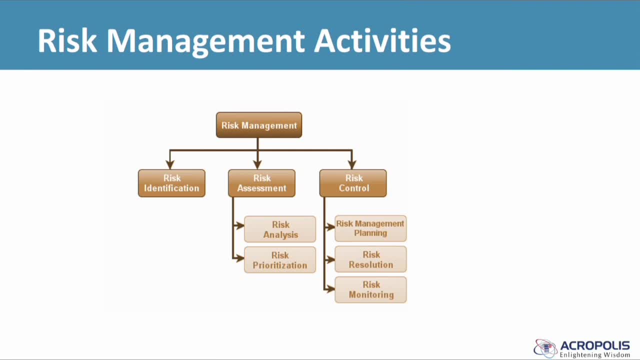 risk management activity. here we have one diagram uh. so the first stage we have this identification, and then a risk assessment, which is subdivided into risk analysis and risk prioritization, and then we have risk control uh. in that we have uh risk management planning, risk resolution and risk monitoring. so let us look uh in detail what we have uh. the first one is: 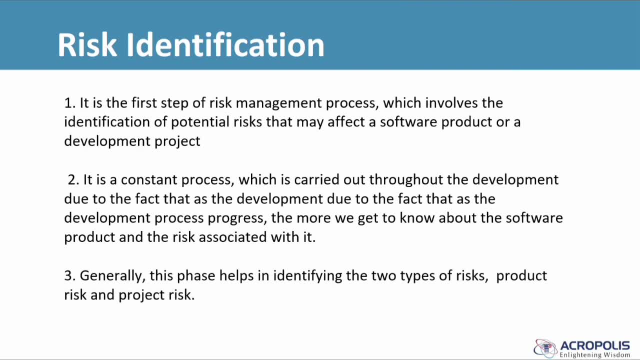 this identification, so it is very first step of risk management process. it generally involves the identification of potential risk that may affect a software product or development project. it is a constant process. it is a constant process that is uh like carried throughout the whole development due to the fact that, as like development progresses, as 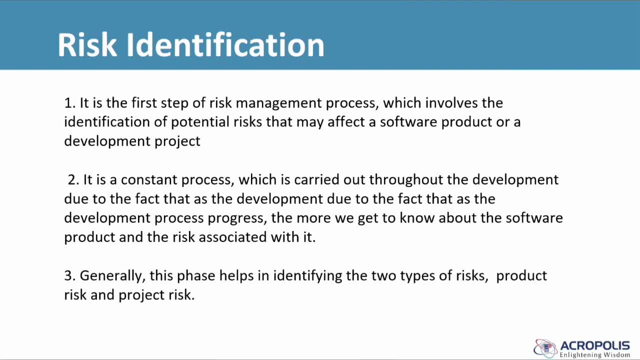 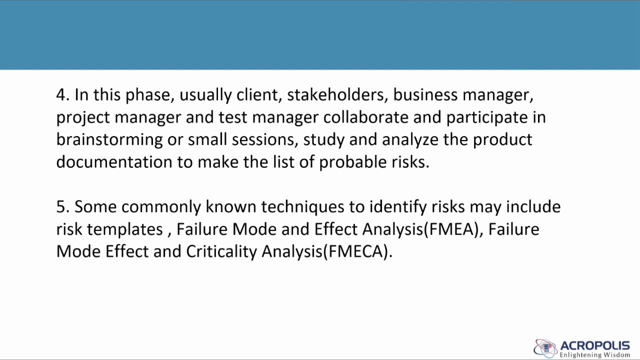 development process progress. then we know about the project, uh like product much better and the risk associated with it and generally this uh this phase helps in identifying the two types of risk, that is, product risk and project risk, right? so in this phase one we generally do usually like we take uh brainstorming sessions or small sessions, uh like. 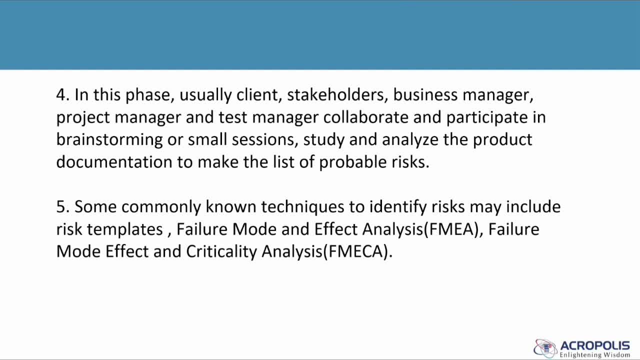 we have client stakeholders: business manager, project manager and test manager. they collaborate and participate in brainstorming session and study and analyze the product documentation to know to and make the list a probable risk. so some common uh techniques that we use to identify risk is uh like failure model and effective analysis, shortly known as fme. 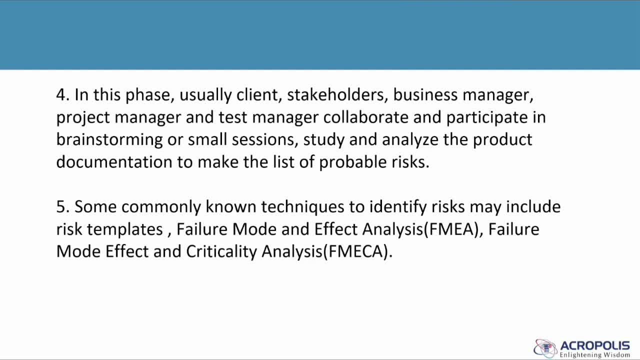 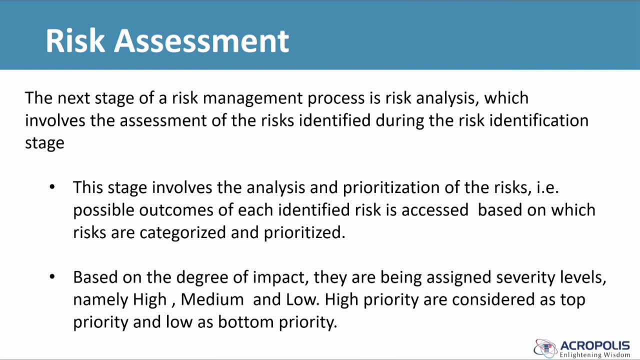 a and uh, failure mode effect and criticality analysis, fmeca. these are some techniques which is used to identify risks. now, uh. after that we have risk assessment. uh, this is the next stage. after this management process, we do the analysis. it is subdivided into two parts. like we analyze. 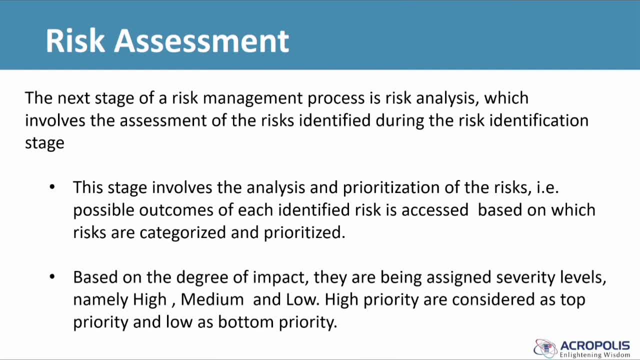 like, we do analysis and prioritize the uh, like how much risk is? so generally, what we do? uh, we like access the risk. we, after identification, we access the risk and then it is categorized and prioritized. if a degree of impact is larger, like, if the degree of impact is larger, uh, then we term. 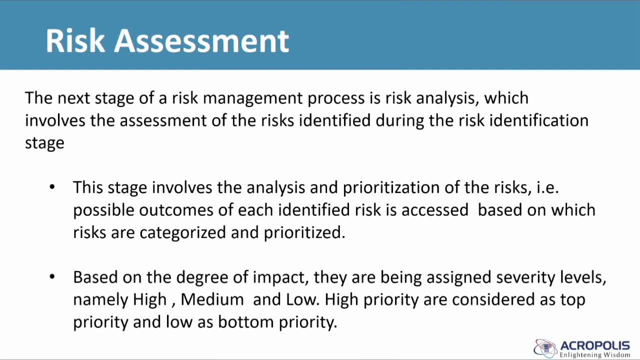 it as high, uh, so far medium and so far low as well, and if the priority of like risk is high, then it is considered top priority and we address it as soon as it is possible. and uh like for low, uh, low, low priority, it is like a bottom priority and uh we. 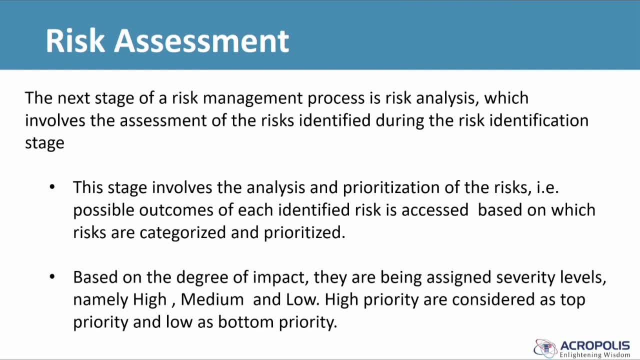 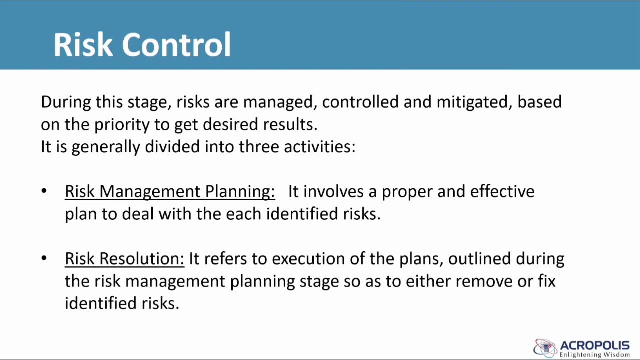 also uh like try to minimize it, but it happens after uh like managing high priority risk. so, uh, now, after this assessment, we have a risk control. so, yeah, what we generally discussed, we discussed uh a risk identify first of all. we like identify the risk and then we categorize. 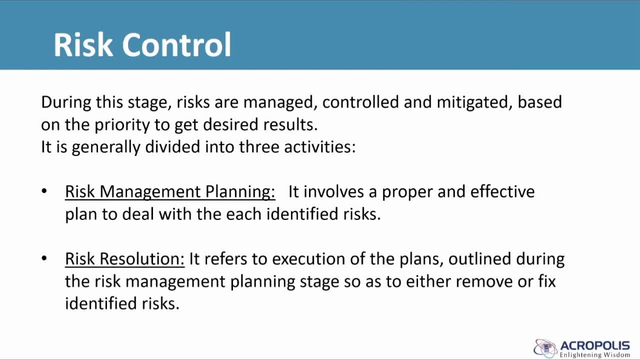 and we analyze and prioritize it and then, after doing that, we will control, we will try to control. the risk associated- so it is generally divided into three activities- is the first one is risk management planning. uh, so like in that we, uh, we, like we come to know, or we.